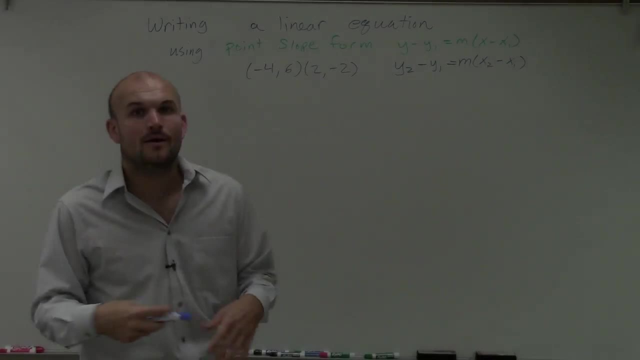 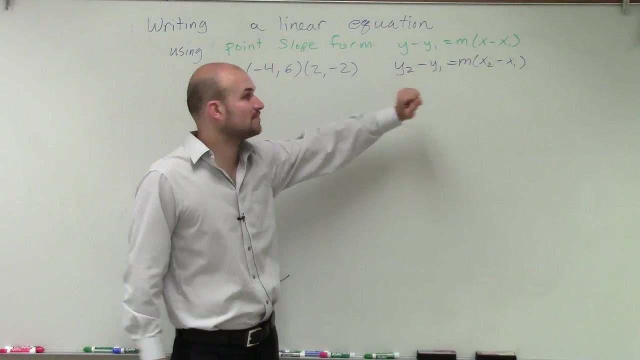 Okay, so what again is we have is we have two points here and we want to write the equation of the line And we're going to use point-slope form because point-slope form can help us use two points. Now, in my last problem, I showed you how to find the slope. 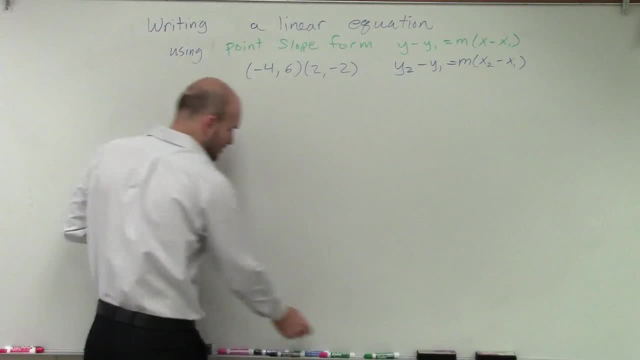 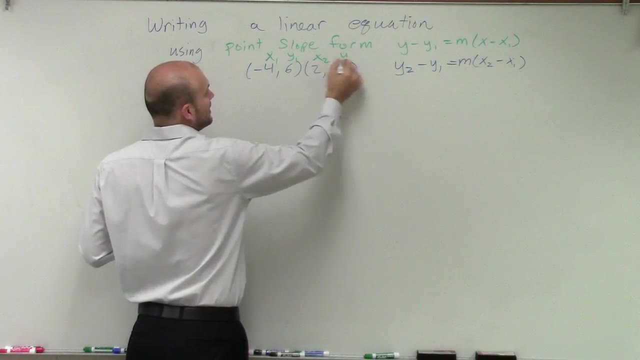 and we could just plug them into the equation. We could also just look at this and say: all right, well, I want to label these. Whenever we have my two points, I know that these are both x and y coordinates and I'm going to label them x1, y1, and x2, y2.. And a lot of. 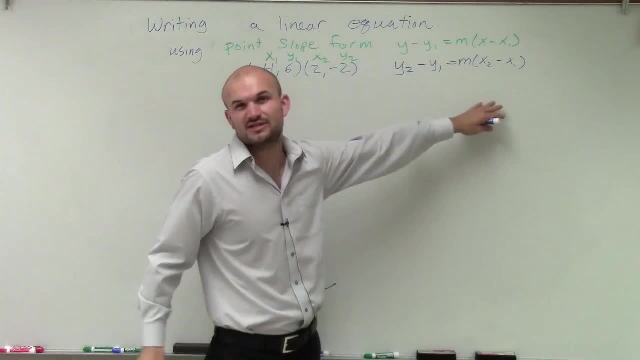 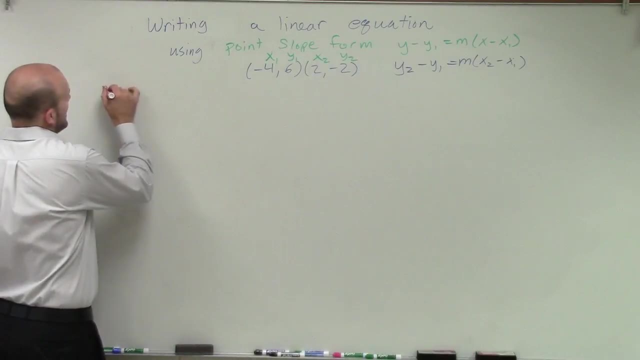 you are probably familiar with the slope formula. So rather than plugging them into this equation and finding the slope, we can easily just write them into the equation of the slope formula. So the slope formula, remember, is m equals y2 minus y1 over x2 minus x1.. So 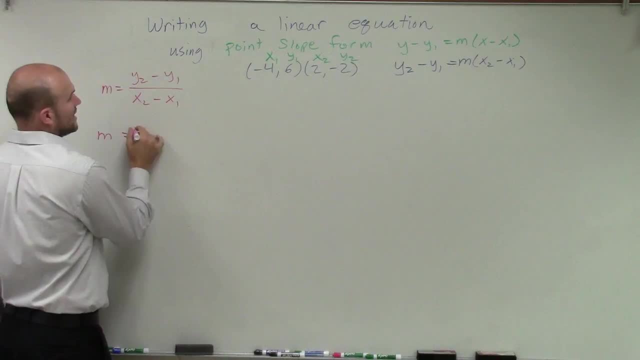 therefore, I'll just go and figure this out here real quick. So I have negative 2 minus 6 all over 2 minus a negative 4. Well, negative 2 minus 6 is going to be a negative 8. And 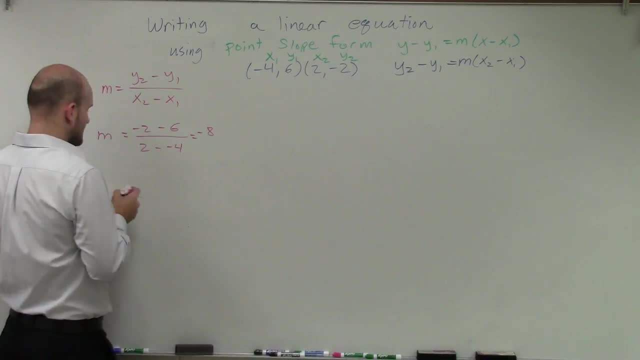 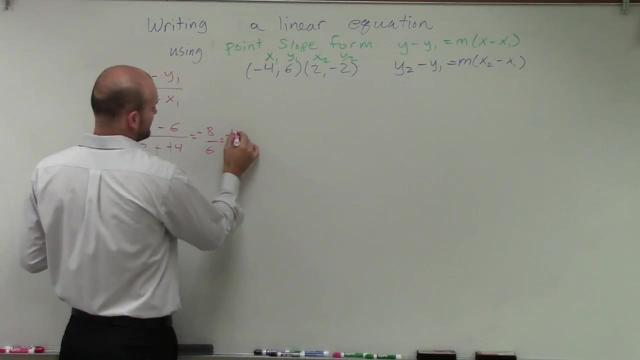 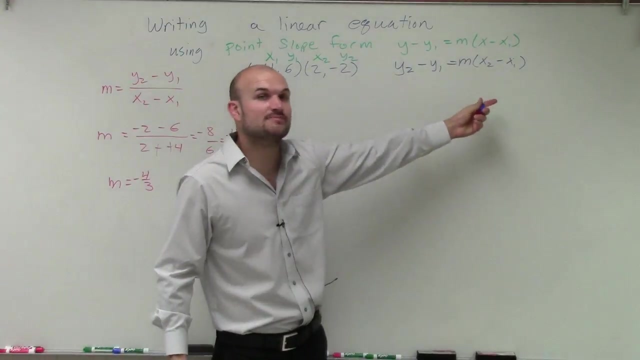 negative 2 minus a negative 4 is going to be a double positive, so that will make it positive. over 6,, which equals divide, you'll have a negative 4 thirds. So now we know m equals a negative 4 thirds. So when writing my equation using my point slope form, I'm 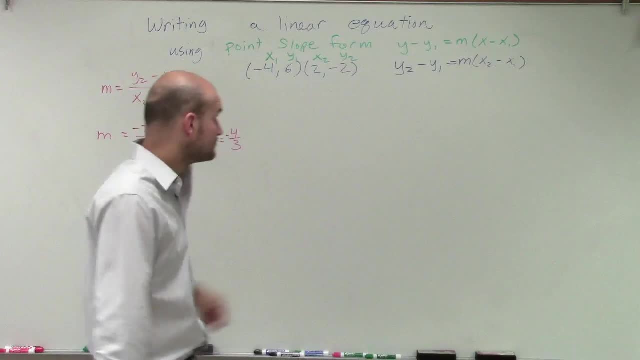 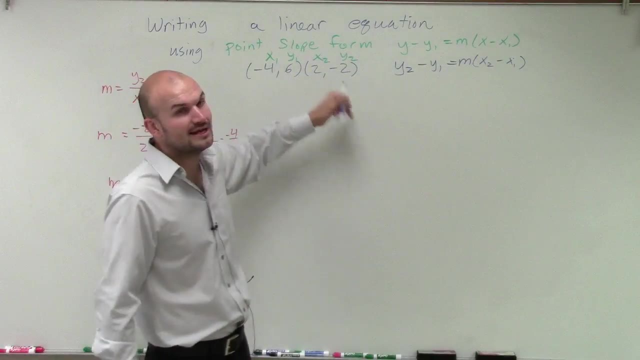 going to now put a negative 4 thirds in for m. But the next thing is, we know that we're going to put that in for m, but then we need to determine, well, what other point can we plug in? Or I showed you how to write it into slope intercept form, where we're just given one. 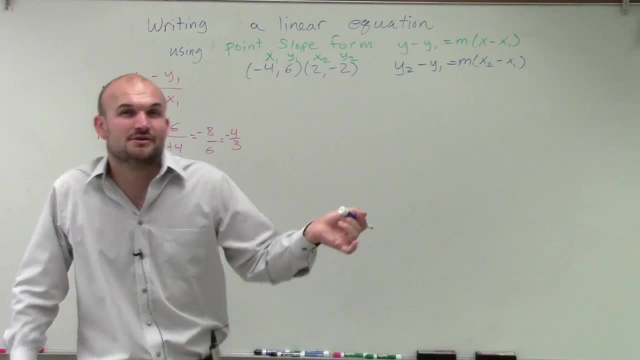 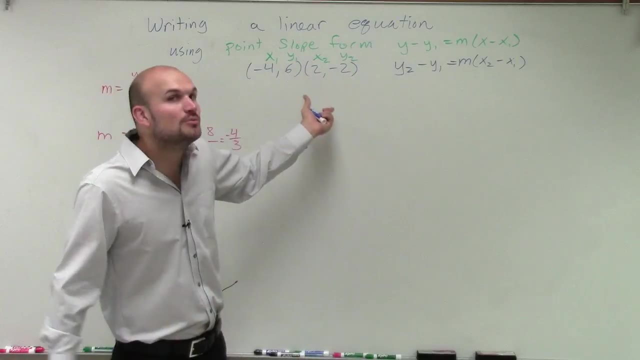 point and the slope. Well, now we're given two points, So we need to determine which point do we pick, And it doesn't matter, because it's going to be true for all points that lie in the line. So, since these are the two points that we're told are on the line, we 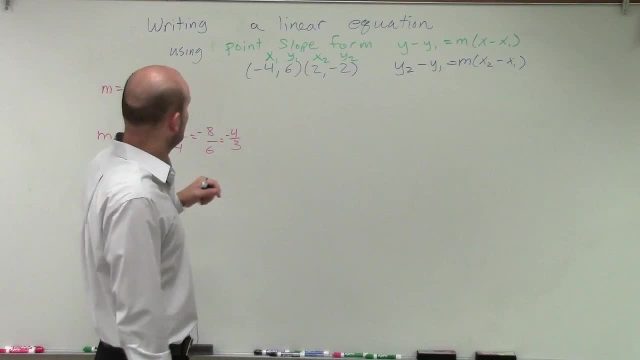 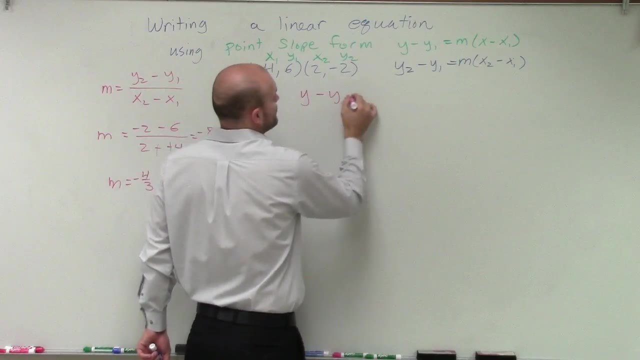 can choose either one, And it looks like to me. I guess it really doesn't matter. Let's do x2 and y2.. So if I wanted to rewrite this equation rather than writing it as y minus y1 equals m times, 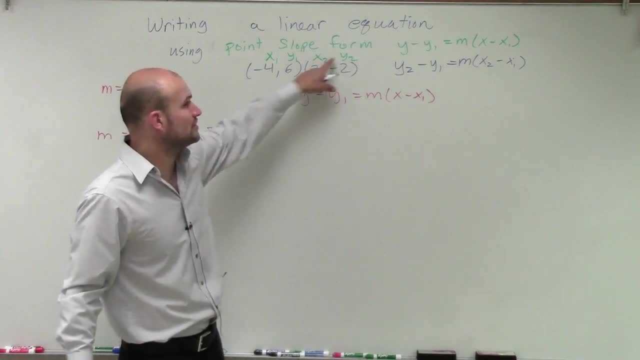 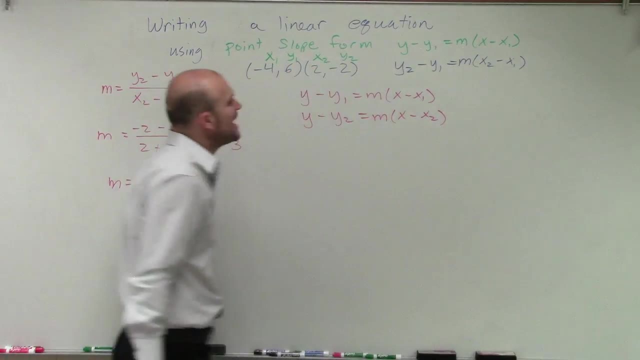 x minus x1,. I know it gets a lot of students confused because they say: well, you're going to use this point. Well then, that's fine, Let's rewrite it like this: It doesn't matter which y's and x's I use, You can just rewrite it, It's going to be.